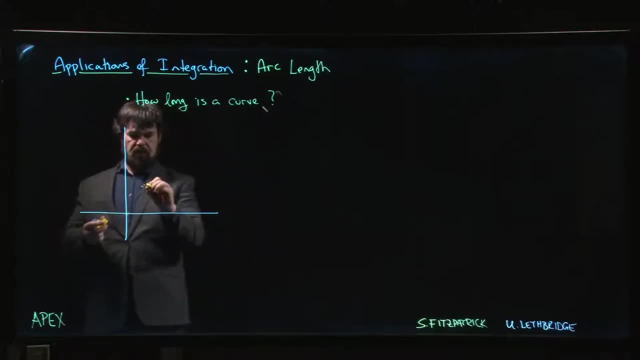 if we have say a point here and a point there, right, And we know the coordinates for these two points. So if this is, say, x1, y1, and over here is a point x2, y2.. Well, we know how to measure. 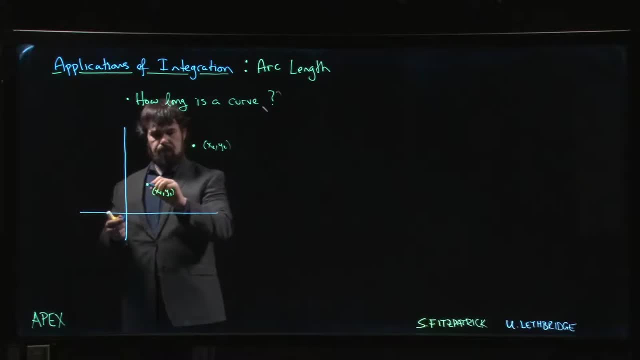 the distance between them. right, We just draw the line from there to there and then we rely on essentially, Pythagorean theorem. right, We set up this triangle. We know that delta x is just x2 minus x1.. We know that delta y is y2 minus y1. And if we have this distance d well, Pythagoras. 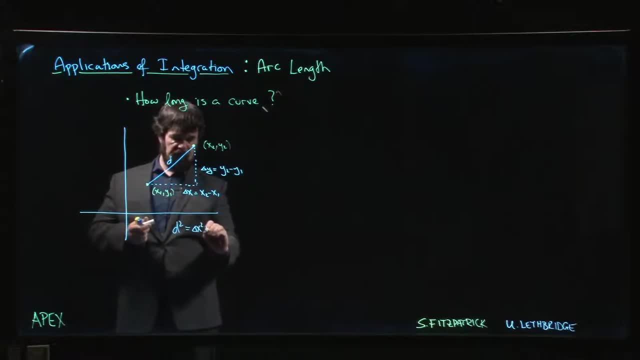 says that the distance squared is delta x squared plus delta y squared. okay, So this is something we understand and we know how this works. Another question is: well, what if you go from there to a situation where you're going between two points but you're not doing it in a straight? 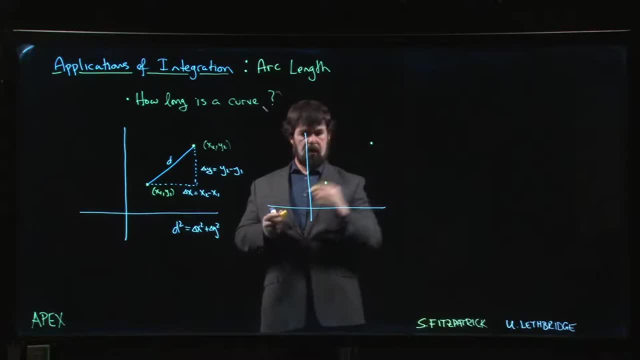 line, right? So what if you're going from here to there and, instead of following a straight line, you follow some curve? Maybe we travel like this. How do we measure the distance now? Well, we fall back to a technique that we've done many times in the past, right? 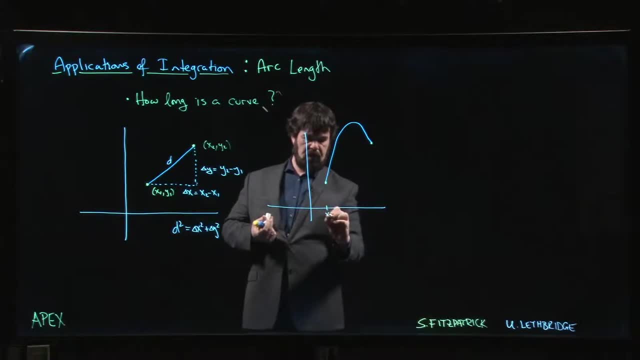 Um, we still start with an initial point x plus 1, right? So this will be: maybe we call this a. We're going to end at some final point b and we're going to call that maybe xn plus 1, and we're going to introduce. 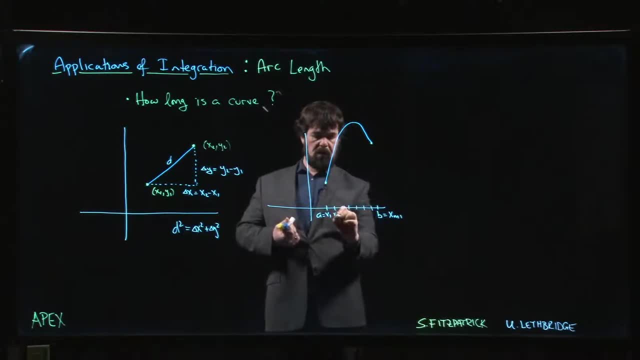 a whole bunch of other points in between: right, x2,, x3,, x4, and so on. right, We partition, And so that partition, well, this is going to be xn plus 1,. right, So this will be xn plus 1, and we're going to call this a. 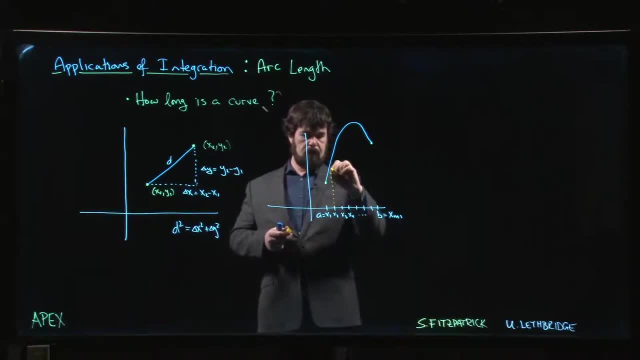 It introduces a bunch of intermediate points on our curve, like so. So it's a very similar picture to the one that we encounter when we're doing, let's say, areas or something like that We partition, But this time we're not going to try to calculate the area of rectangles or do anything like. 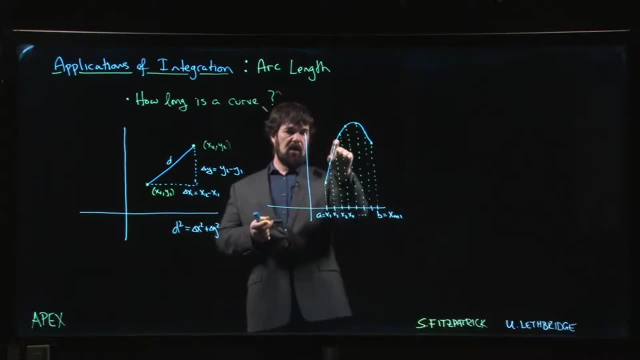 that. Instead, what we're going to do is we're going to calculate the distance between points, And for portions of the curve where the concavity is small, as measured by the second derivative, this works pretty well. The deviation from a straight line here is not that significant. 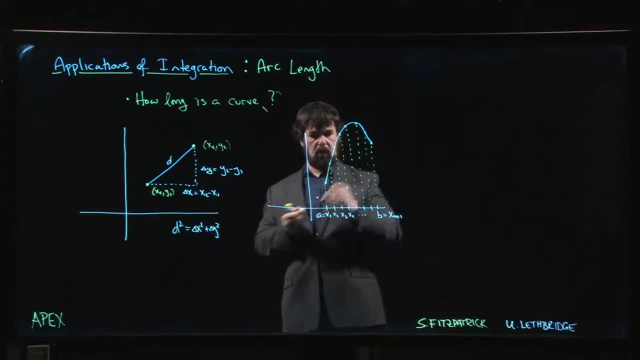 Same thing here. So let's try this and maybe white will work better. There, there, there we see a bit of deviation and there, there it's more significant. there it's more significant, and there. But this sort of piecewise linear path. 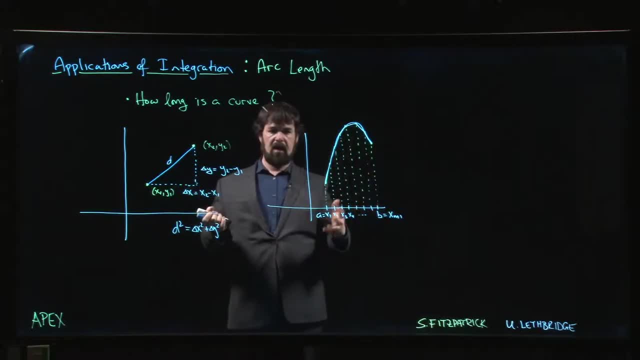 It's a reasonable approximation to the original path. And as you take more and more points, the approximation gets better and better. And so this distance that we're interested in, this length of the curve, the length that we're interested in, well, it's approximately that first distance squared plus the second. 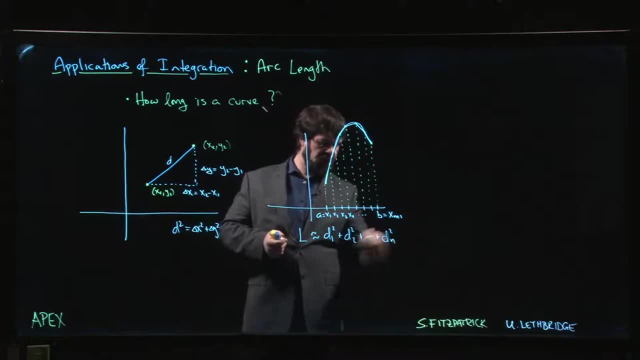 distance squared down to the last distance squared Where, At each of these distances? well, we can say exactly what it is right, D i is going to be the square root of delta x- i squared plus delta y- i squared right. 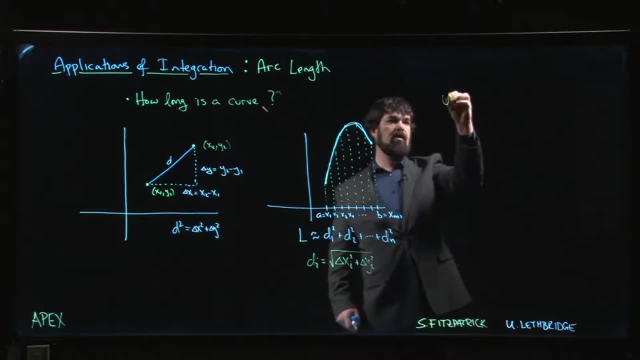 And probably you want to do a uniform partition. That's sort of standardized. So we're going to do a uniform partition. OK, That's sort of standard practice for us, right? So if we're doing a uniform partition, then we know that delta x- i should just be delta. 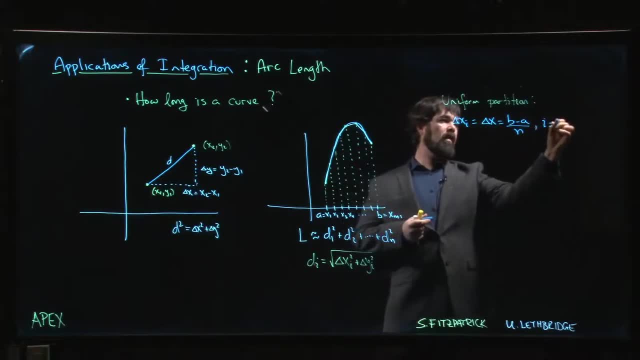 x, our usual b minus a over n for each i, going from 1 up to n. OK, What about delta y i? Well, delta y i is going to be f at x i plus delta y i, squared, So it's going to be f at x i plus- oops, sorry, should be in the subscript: i plus 1, right. 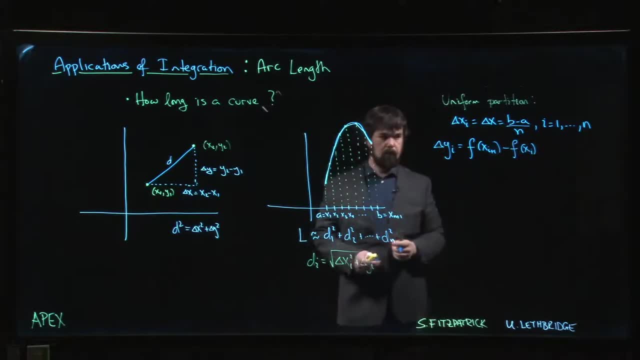 minus f at x. i OK for each, i OK. So we can kind of put that together. We can sort of put this as a Riemann sum. But actually there's a thing we can do Which is even better. 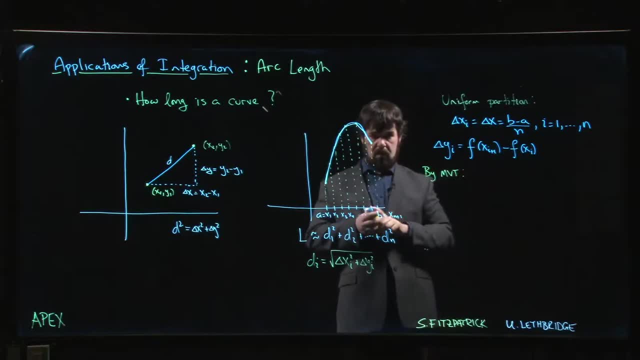 By the mean value theorem. I can take this difference and I can write it as: and now, of course. now I have to assume that my function is differentiable, continuous right. So, and of course, if it's at least continuous right, maybe there's some points where it's. 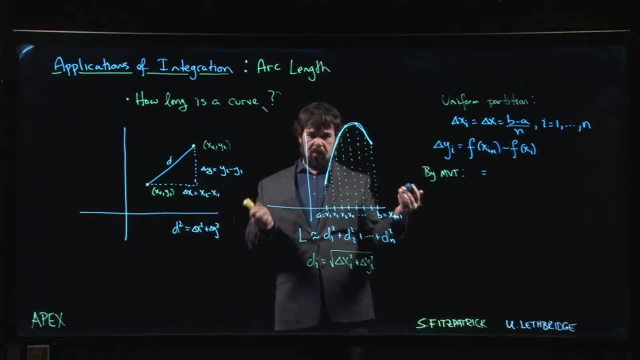 not differentiable, But those are typically going to be custom Cusps, corners, things like that, And we can still calculate the length by breaking, you know, the curve up right If it's continuous. but it's not differentiable. it's probably at least piecewise differentiable. 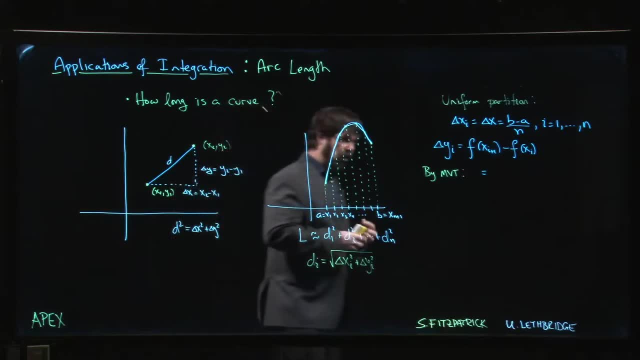 I mean probably. I mean you can construct curves that are continuous everywhere but differentiable nowhere. Really bizarre objects you might encounter in like an analysis course later in your life, But for the sort of things you encounter in calculus typically worst case scenario is: 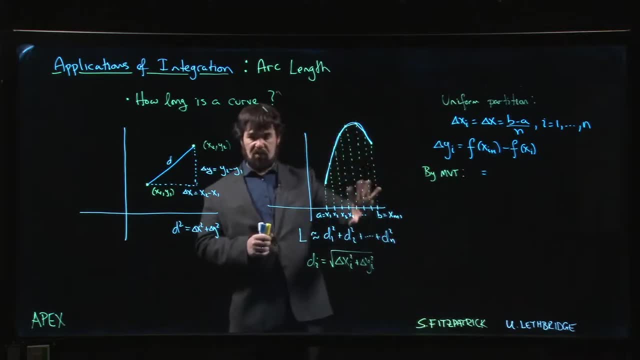 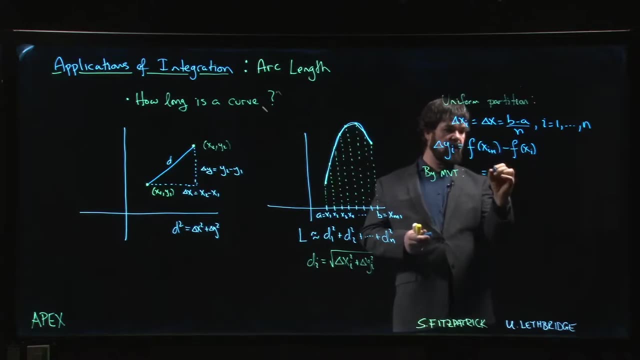 it's piecewise differentiable And you can apply this picture to each part. So if we assume differentiability, then the mean value theorem guarantees that we can write this difference as f prime at some ci times. well, the difference between xi plus. 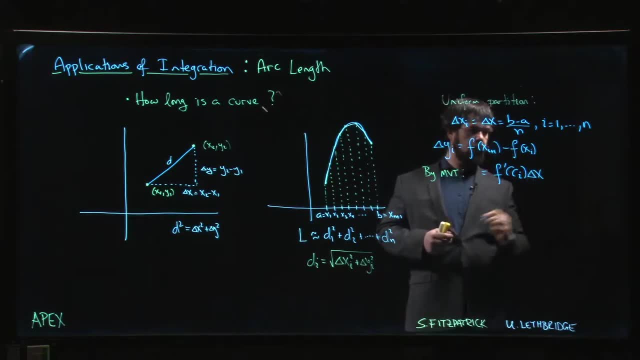 1 and xi. But that's just delta x, Right? So we get delta x, And so ci here. Well, ci is some number between x and x, Right? So we get delta x, And so ci is some number between xi and xi plus 1..